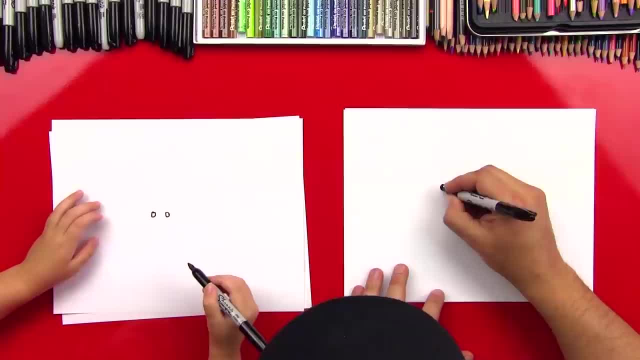 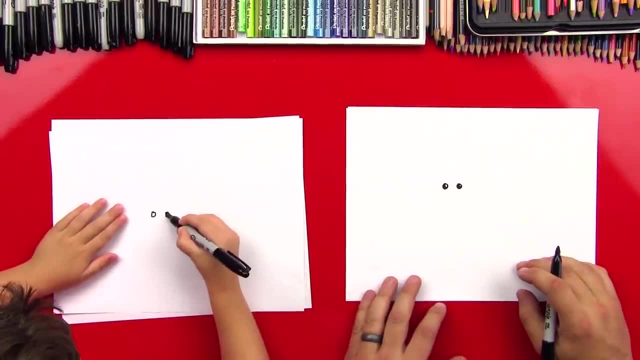 Yeah, good job. And then let's color it in, and I'm going to leave a little white spot in mine, But we can color the whole thing in if you want. Okay, Good job. Oh, I like it Perfect. 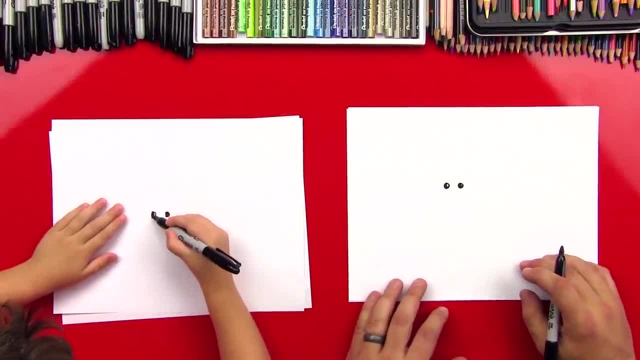 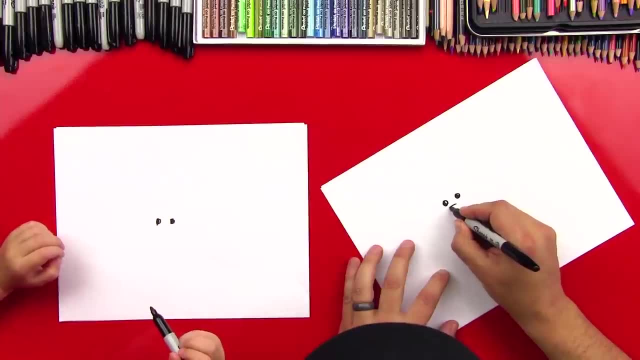 Perfect, You want to do the other one? Good job, man. Okay, let's do his nose next And we're going to do a little oval. okay, We're going to do a little oval right below his nose or right below his eyes. 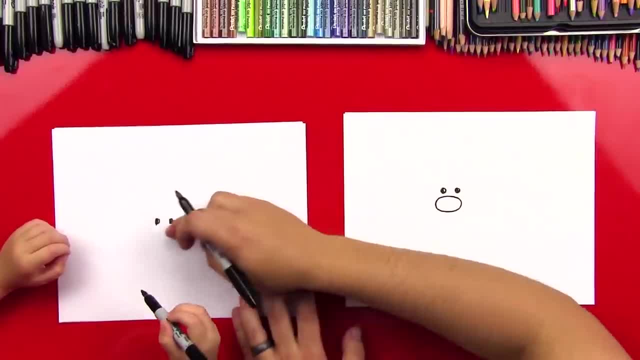 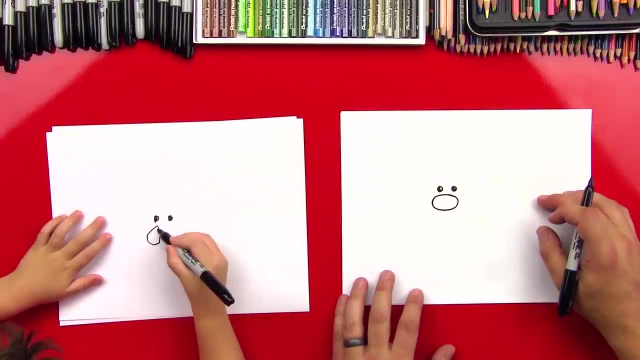 What? Um this one, A big oval right here, Do a little oval. It's kind of a little oval, huh Like a mouth. Yes, Good job, And then we're going to draw his nostrils in there, okay. 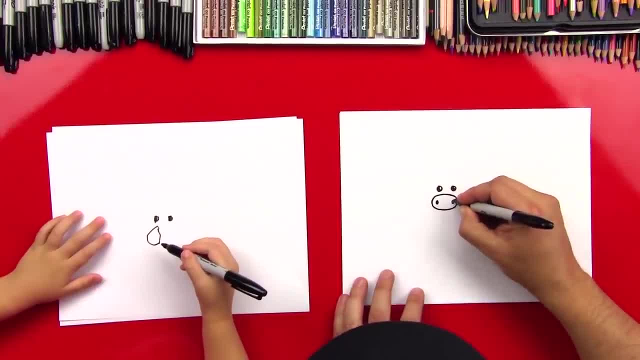 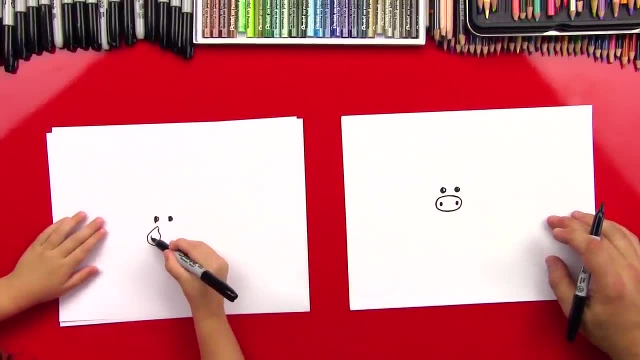 Okay, You can see his nostrils. So we'll draw two little circles or little ovals on the sides so we can draw two little guys right inside there. Okay, His nostrils, Good job. And then one more. 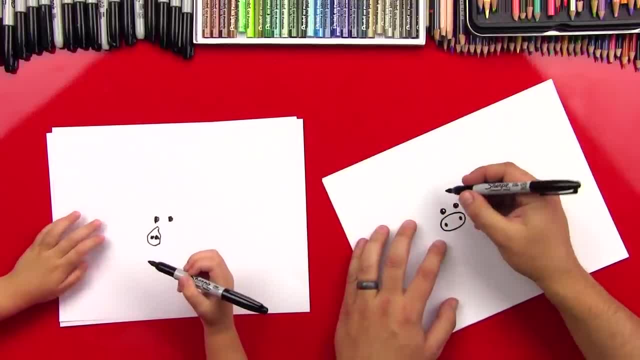 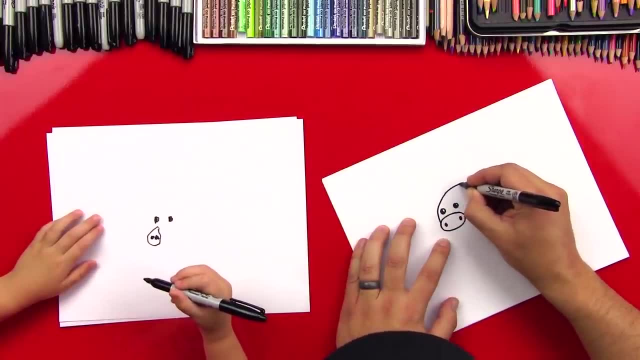 Perfect, You did it. Okay, you ready for his body? Yeah, Alright, let's do it. So this one's going to be a big oval. So we're going to start here, on his nose, We're going to go over his eyes. 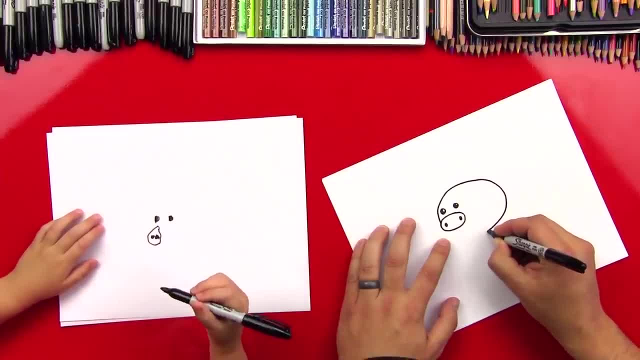 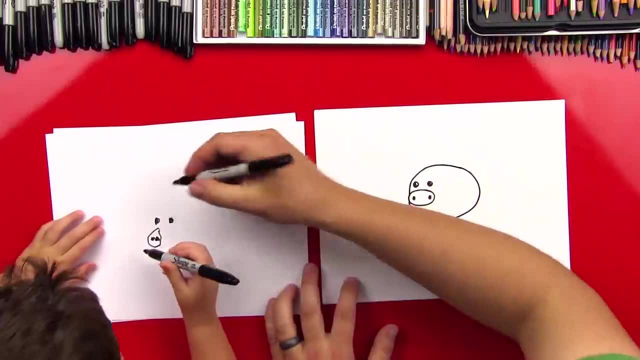 And we're going to come all the way over here And then back And then come back to his nose like that Big pig. So you can start right here, go all the way around, come back and then end right there on his nose. 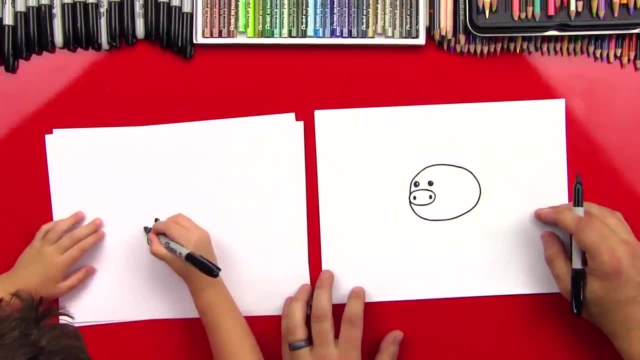 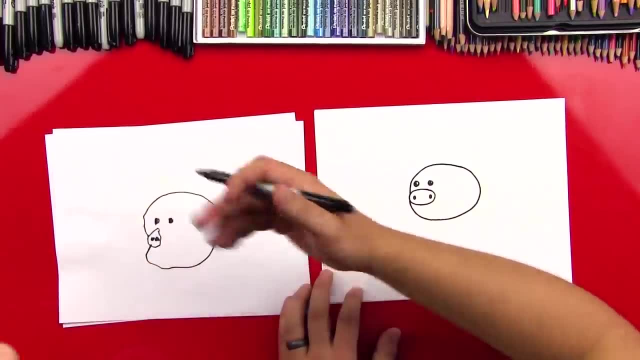 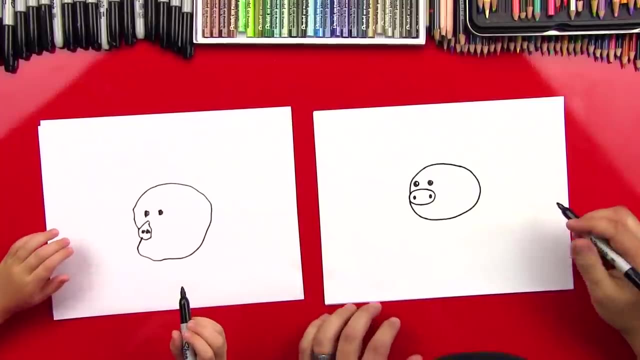 Okay, Okay, let's see ya. Yes, Perfect, That's awesome. Give me five, dude. That's so cool. you did it. Okay now. Mine looks funny, Yours looks funny, I like it, Okay. Okay, now let's draw his legs, Okay. 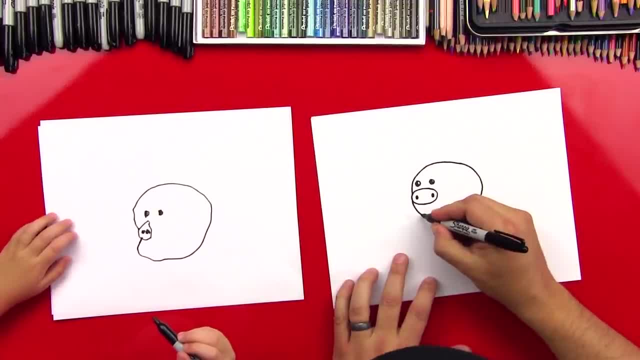 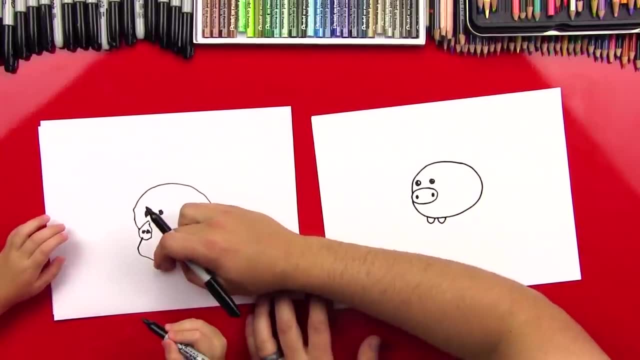 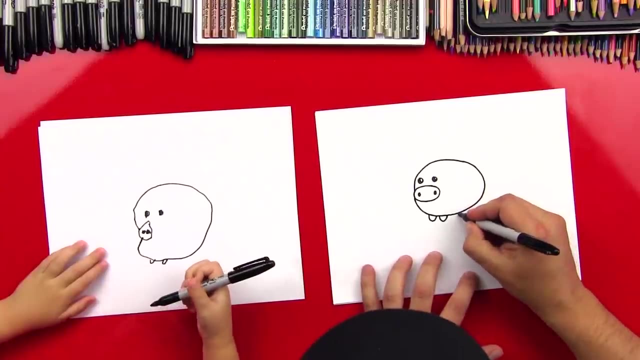 We're going to draw little U's, A U shape. So we're going to draw a little U right here, One, And then we'll do two. One right next to each other. One, two, One, Two, And then let's draw his back legs too. 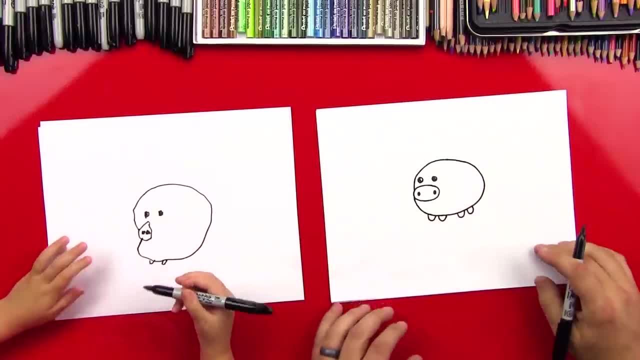 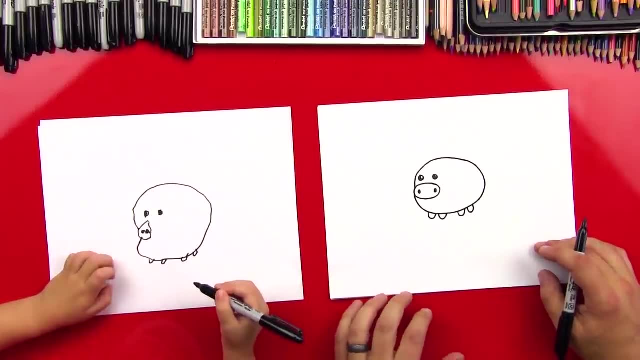 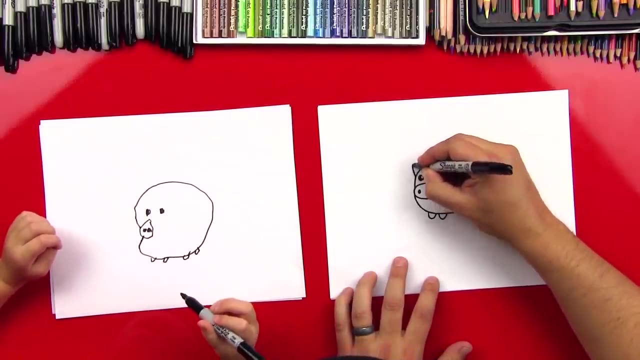 We're going to do little little legs for those too, Okay, Good job. Okay, what's he missing? Ears and his tail. Yeah, Alright, let's do his ears first. So we're going to do a little triangle or an upside down V, okay, 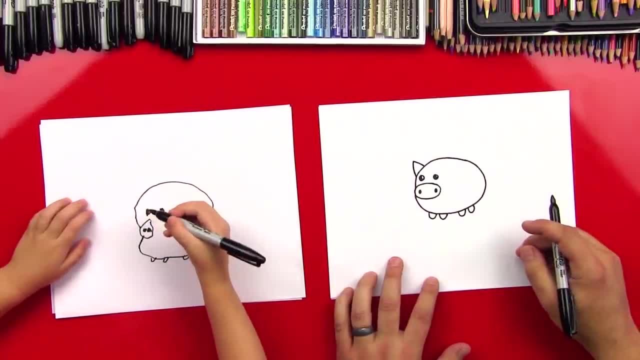 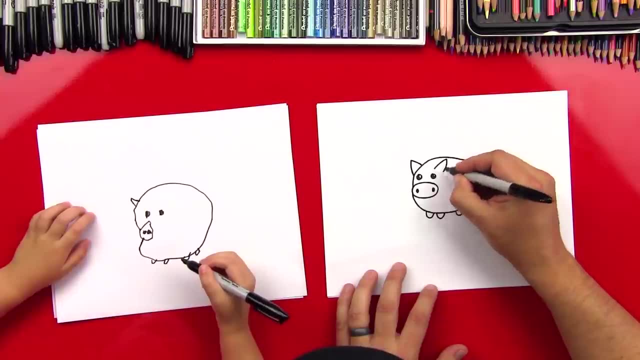 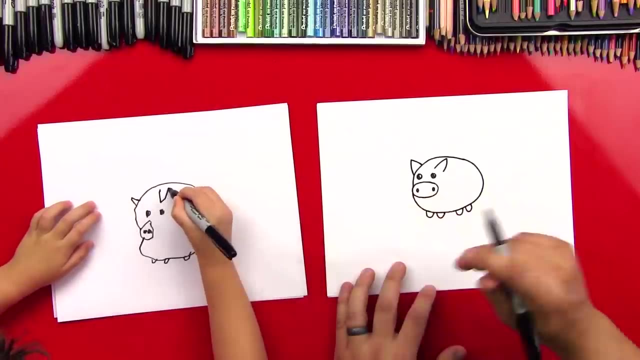 Okay, So we'll do a little V right there for his one ear- Yes, right there, Up and then down. And then we'll do another ear over here, Up and then down, Inside Inside his body- yes, Yup, and then. 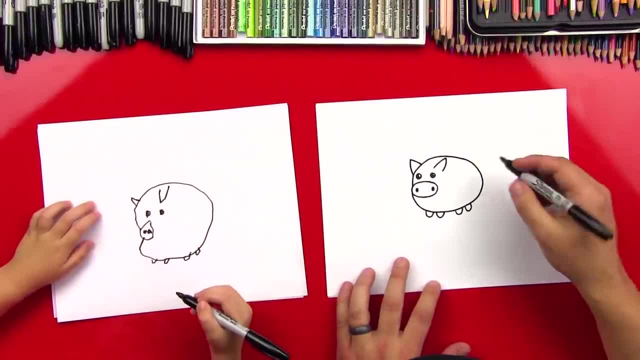 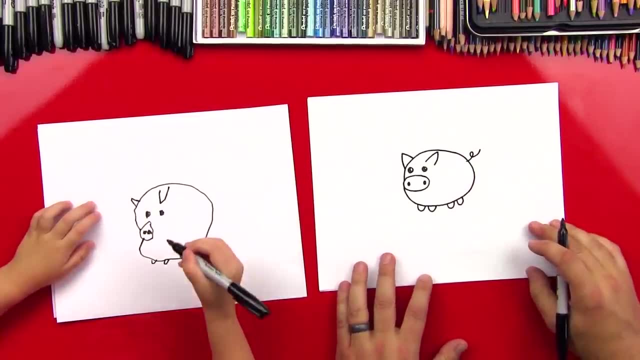 Oh, I like it. Your ear's kind of pointing down- Awesome, I like it. And then let's do his tail next. okay, We're going to do a little curdle like this for his tail. Okay, Because pigs got little curly tails. 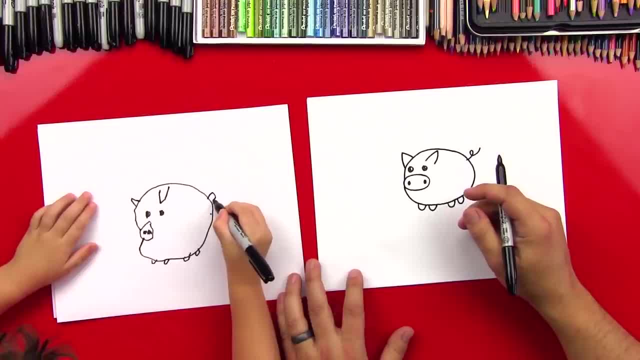 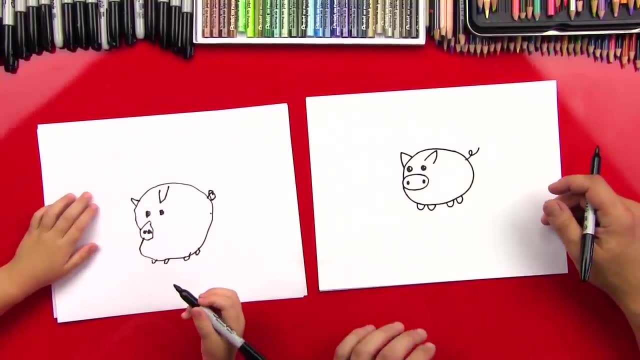 You just do a little loop, There you go, And then, yeah, You did it. What are you talking about? That looks perfect. I could do it. You can do it. Yes, you can. Alright, we need to color him, don't we? 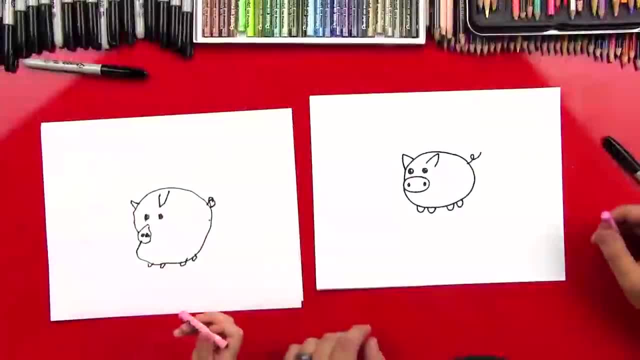 Yeah, Yeah, what color is the pig? Pink, And then we'll color him in. Alright, Austin, we're just going to use one color. We're going to color the whole pig in. okay, Should we fast forward? Yeah, 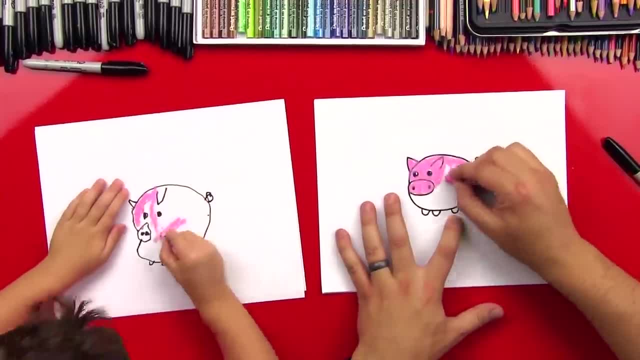 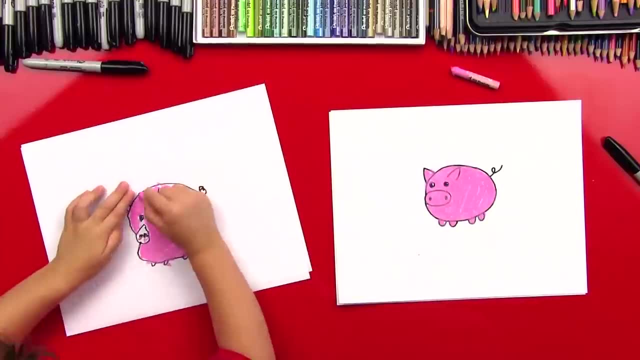 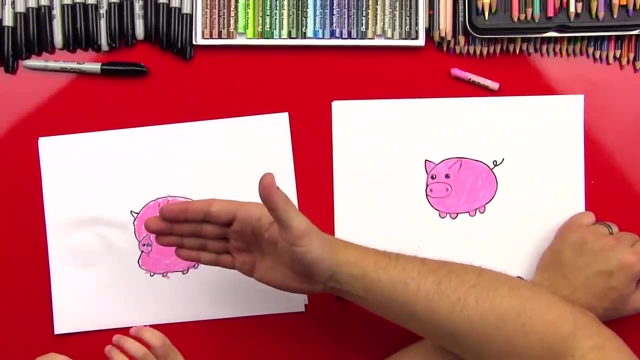 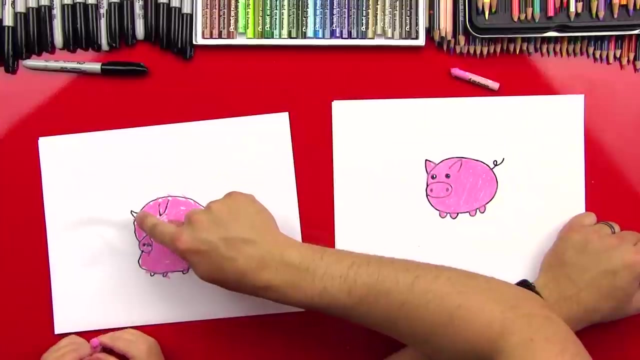 Alright, let's do it right Now. Austin, good job, man, You did such a good job. I really like your pig, You promise. Yeah, He looks really cool. You can also color his little ear right there. 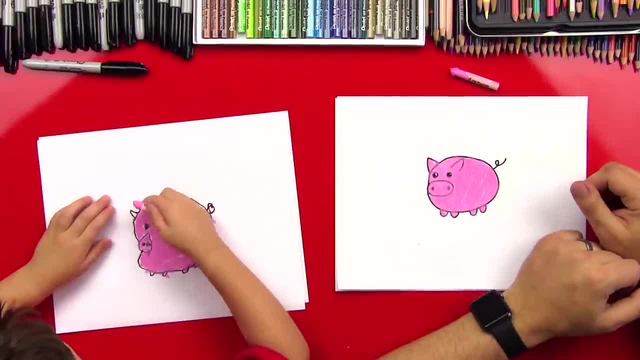 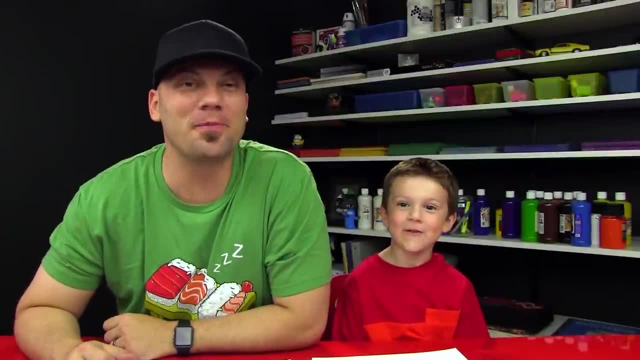 You want to color his ear? Oh yeah, Oh yeah, You did it: You colored his ear. Good job, man. We hope you guys had a lot of fun drawing and coloring your little pigs with us Right Austin. 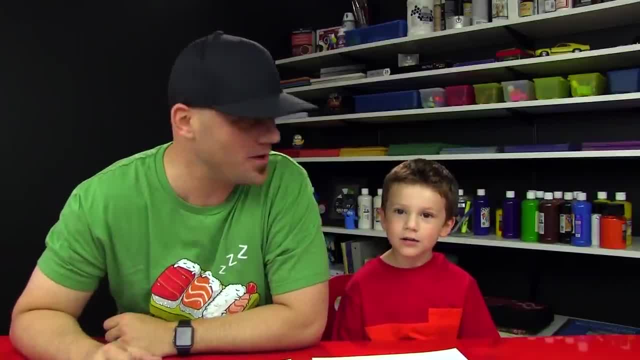 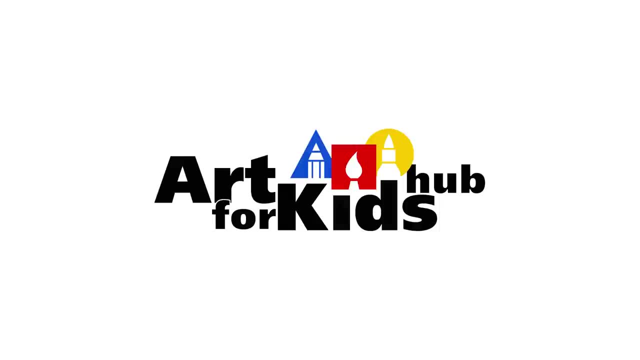 Yeah, Yes, this activity was meant just for little artists, so we hope you guys had a lot of fun. We'll see you later. huh, Yeah, Should we say goodbye? Yeah, Goodbye, Bye-bye.